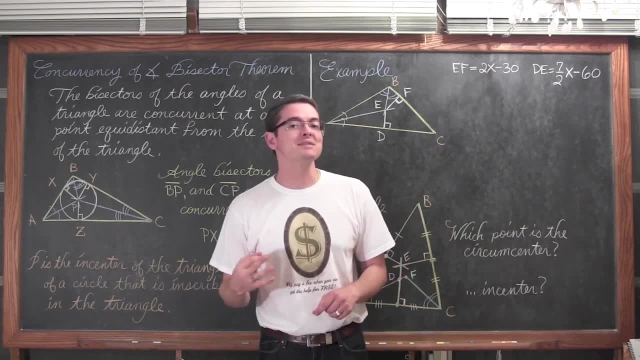 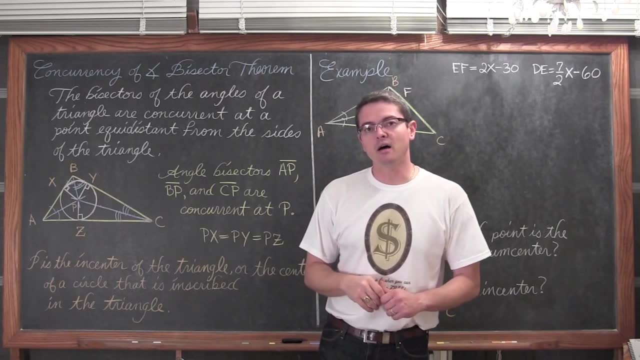 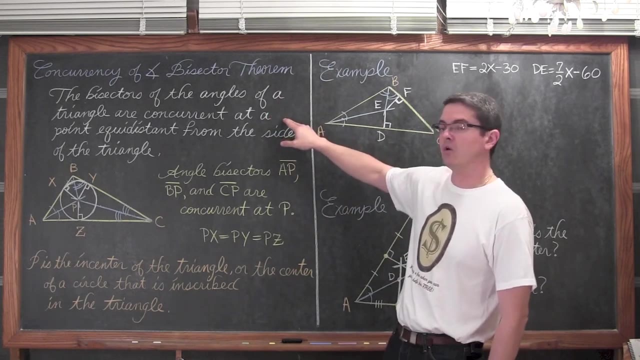 of our three perpendicular bisectors was the circumcenter, or a point which was an equal distance to the three vertices of the triangle. Now we are going to be talking about angle bisectors. The bisectors of the angles of a triangle are concurrent. remember that is. 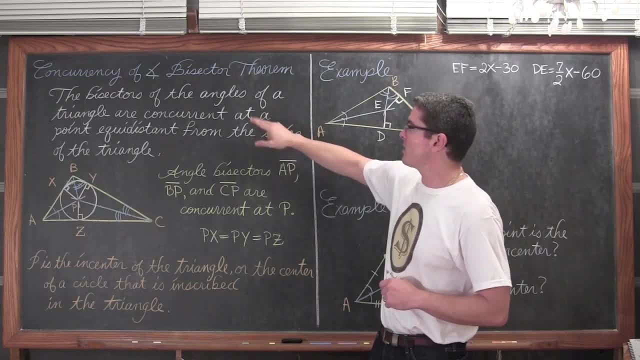 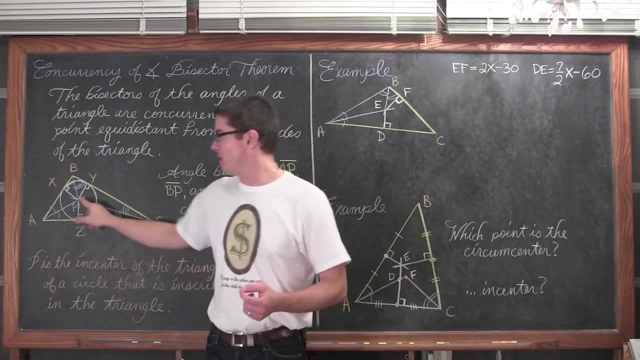 three points or more intersecting at the same point are concurrent at a point, equal distance from the sides of the triangle. So instead of our concurrency point being an equal distance, an equal distance to the three vertices, again like the perpendicular bisectors, this concurrency. 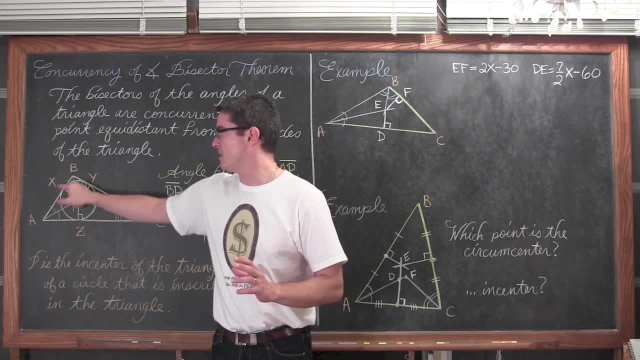 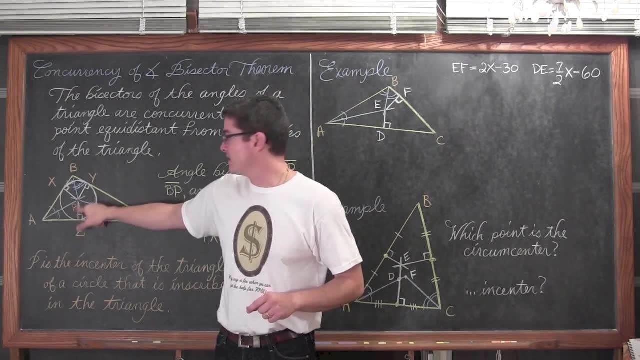 point is going to be an equal distance to the three sides of our triangle. Let's not forget that we measure the distance between a point and a line in a perpendicular fashion. So we go from a point P to Z in a perpendicular little segment, and from point P to Y and P. 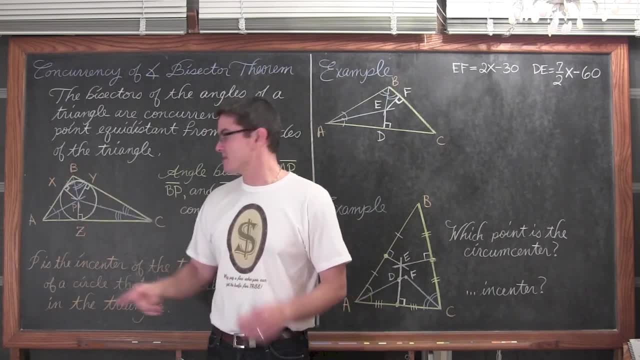 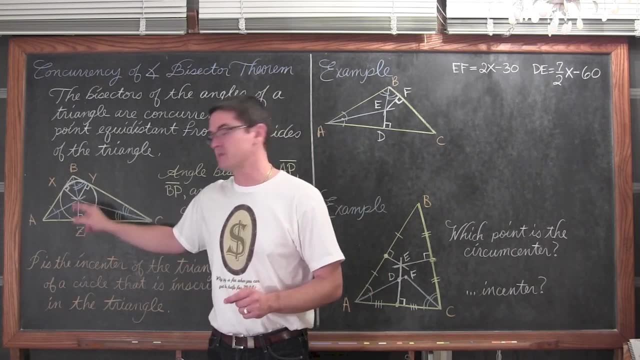 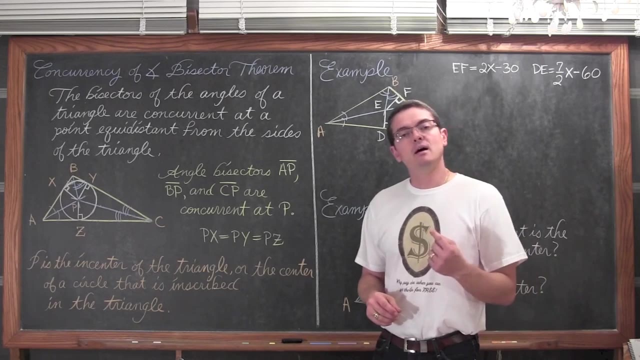 to X, All perpendicular. That means that these three segments are all radiuses of a circle. Now the circle can be drawn from this point of concurrency, which, by the way, is called the in-center. Point P is the in-center of the triangle where the three angle bisectors intersect, Or the 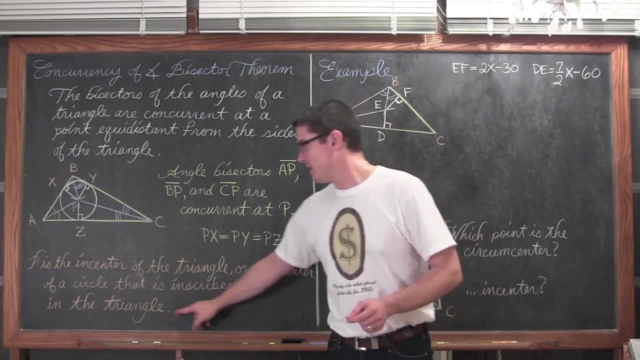 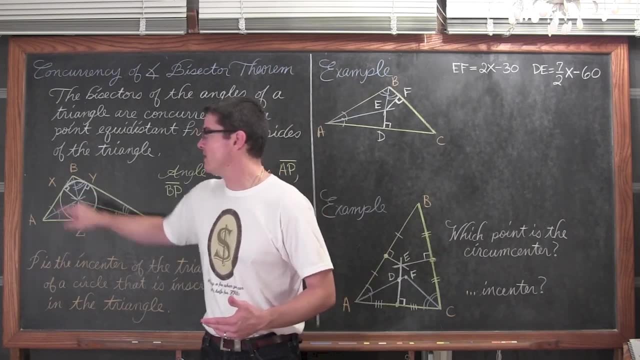 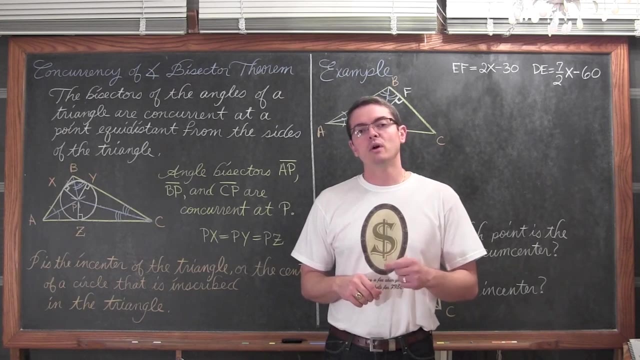 center of the circle which is inscribed in the triangle. So we have three angle bisectors. we got point P, the point of concurrency. boom, There is an in-center, There is an inscribed triangle, Again, unlike your perpendicular bisectors which meet at 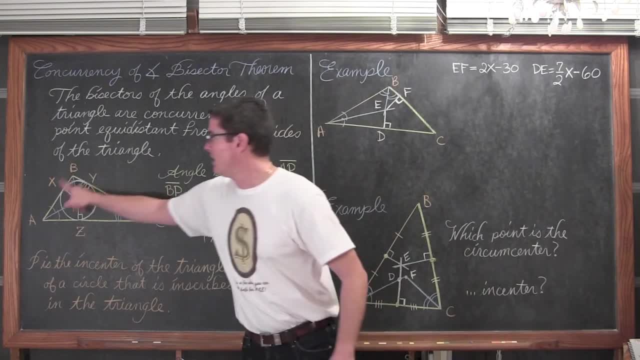 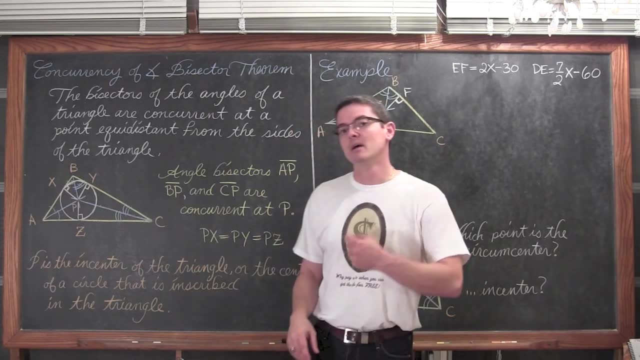 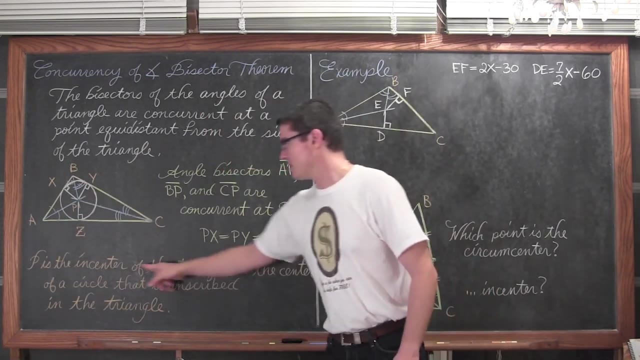 the circumcenter of the triangle or the center of a triangle which can be. my hand motion is making a very poor circle, but can circumscribe the triangle. The angle bisectors point of an inscribed triangle or the point of concurrency is again the in-circle. Ok, we are only going. 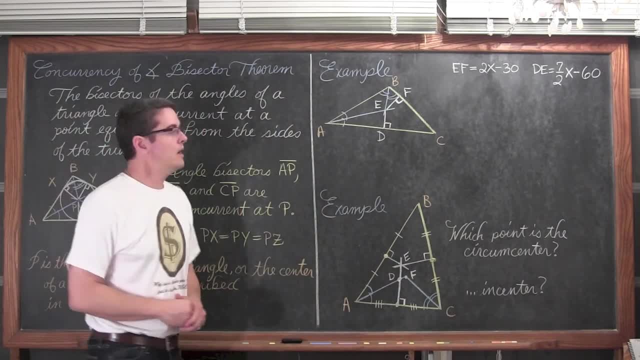 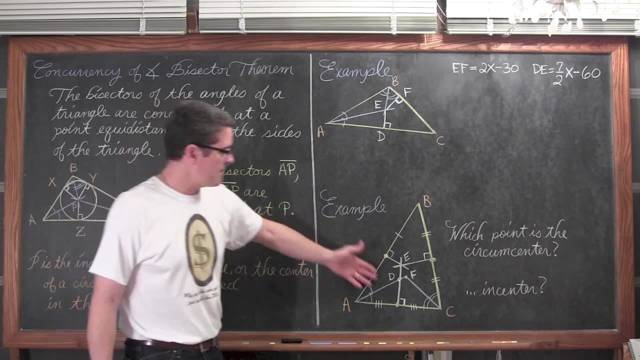 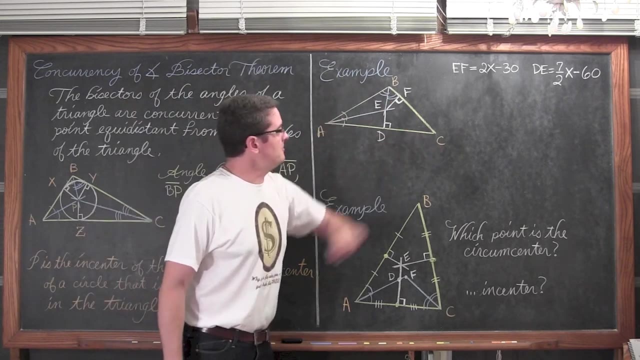 to do a couple of quick examples. We will prove this later on in the year. Therefore, our examples are going to be just two, One algebraic and one identifying the type of point where some bisectors are meeting. So we have triangle ABC and we have an angle bisector here of AE and an angle bisector. 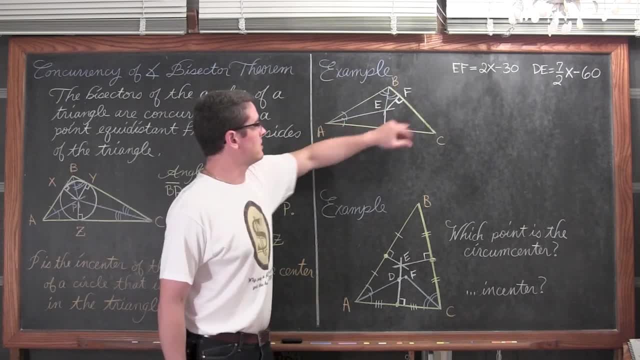 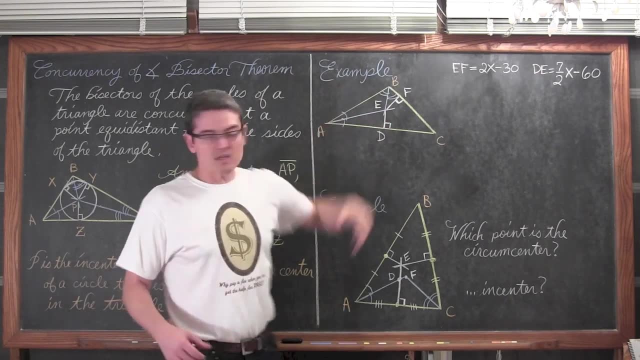 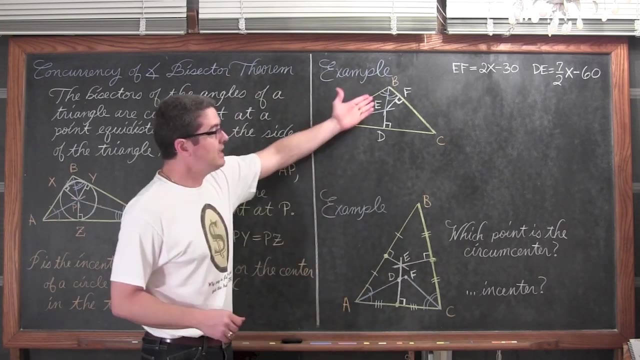 of BE. These can be either lines that are intersecting the angles or rays. We have a point of concurrency here Now, If we just learned that the three angle bisectors all meet at a common point. this point of concurrency I do not need- though I could, I do not need to draw all three angle bisectors. 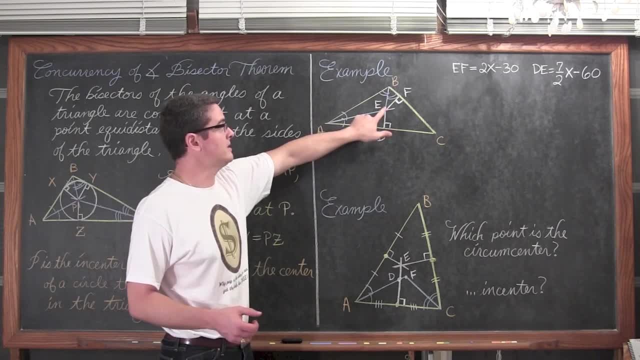 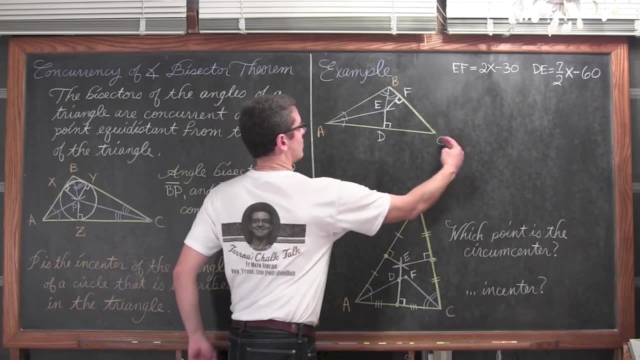 to identify this point E as some kind of special point. It is the intersection of two angle bisectors and thus from this it is going to be the intersection point of actually all three angle bisectors. But I have got two angle bisectors, I have got E. This is the 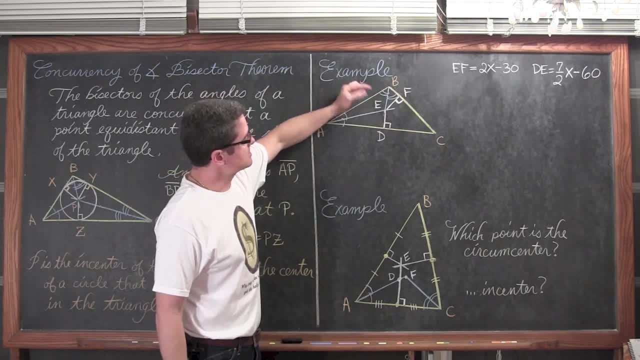 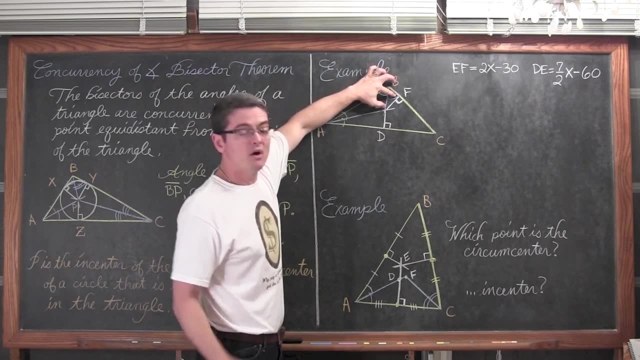 end center of this triangle, which means that this perpendicular length going to the side of the triangle ED is going to be equal to the length of EF Also approaching the side of the triangle in a perpendicular fashion. If there was no right angle here, then these: 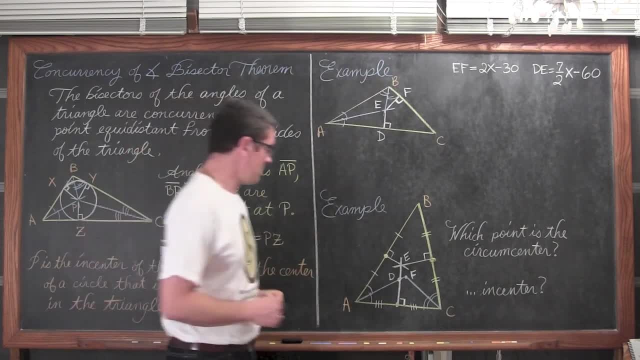 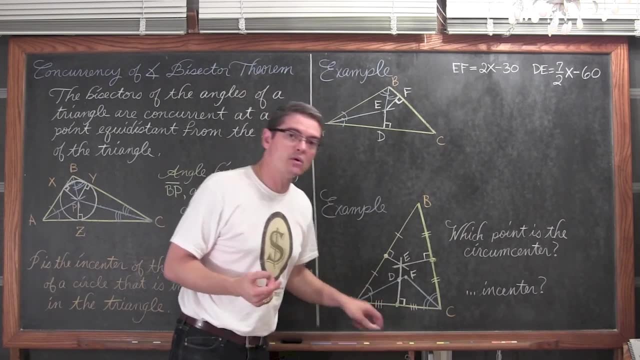 two segments would not be equal, But they are. So they are both radiuses of the end center. Well, since they are equal, that tells us that is exactly how we are going to solve the problem. So if we are told that, 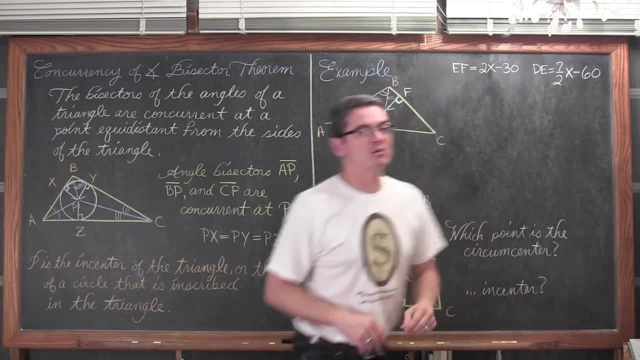 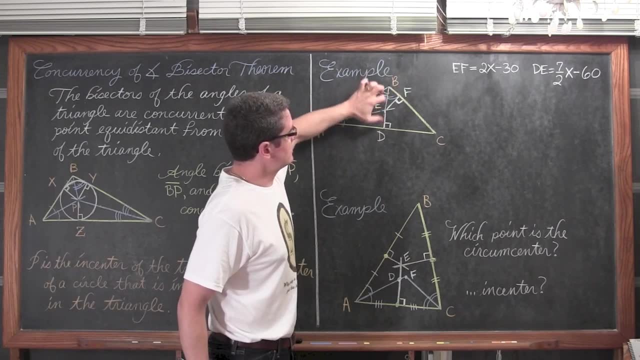 EF is 2x minus 30 and DE is 7x, or 7 over 2x minus 60. Well, if we know they are equal, then knowing that they are equal, being able to say that those two lengths are equal to. 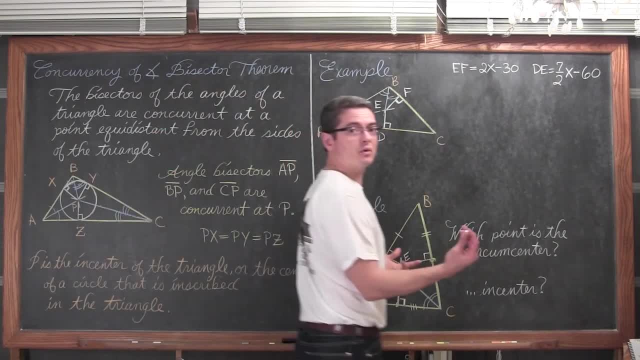 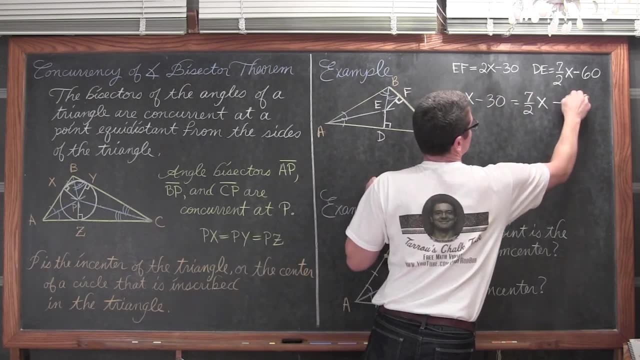 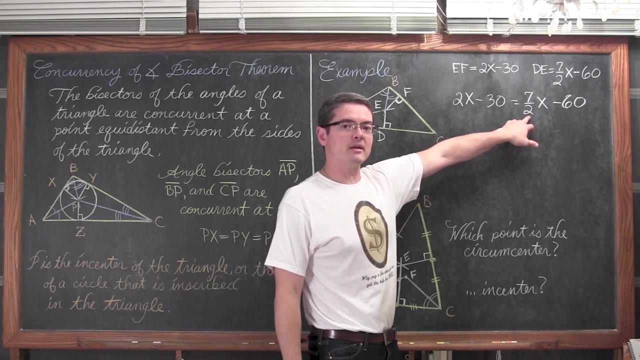 each other tells us exactly how to solve the problem. They are not equal to each other. So we have: 2x minus 30 is equal to 7 over 2x minus 60. We can get rid of this fraction right at the very beginning of the problem by recognizing that we have a division of. 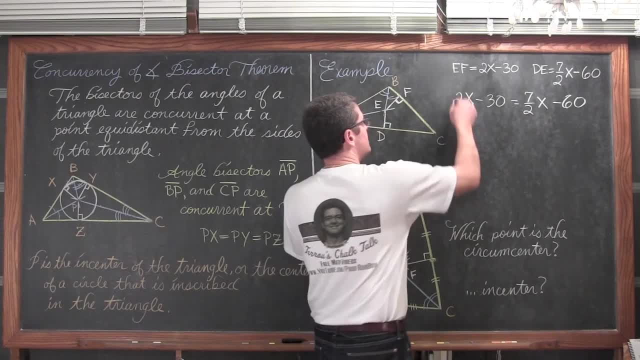 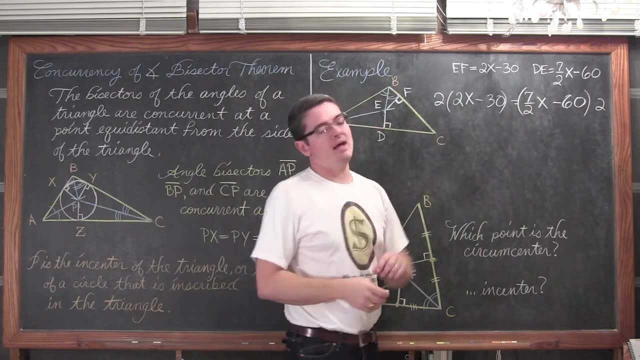 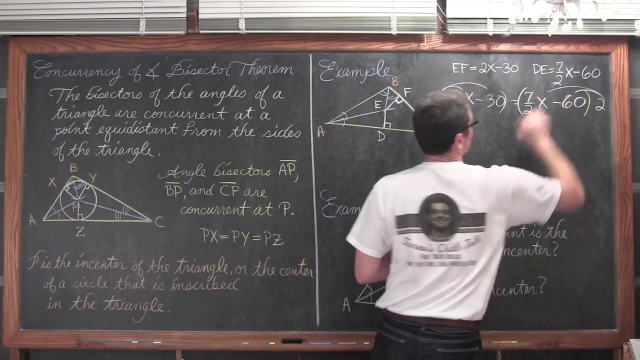 2, and the opposite of dividing by 2 is multiplying by 2.. So if I take a little bit of extra work to multiply both sides of the equation by 2, I will not have a rational value or a fraction in my equation. So I am going to multiply every single term by 2.. We have 2 times 2. 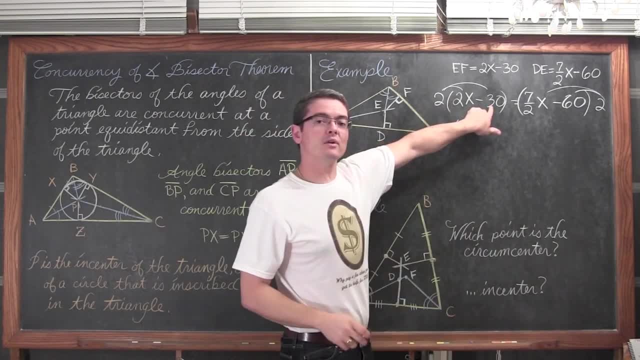 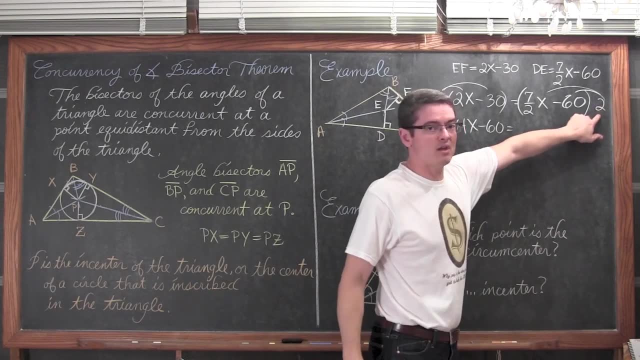 is 4x. 2 times 30 is 60,, so negative 60. This is the minus sign right there. So we have a multiplication of 2 and a division of 2. That is going to cancel out, Or 2 times 7. 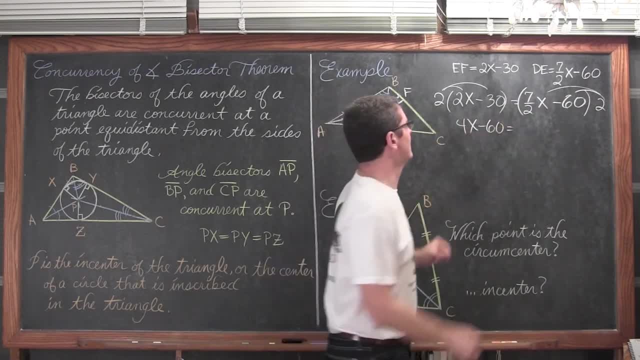 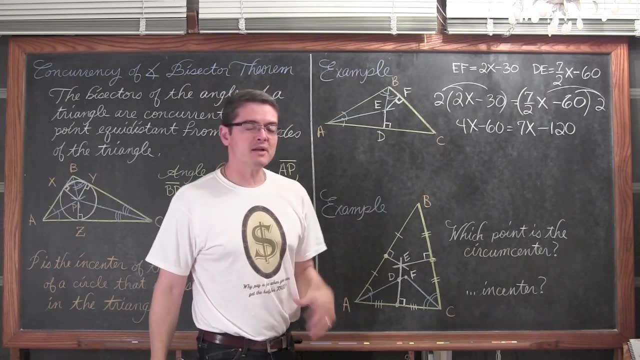 is 14, and 14 divided by 2 is 7.. So we have 7x minus 120.. Ok, we are trying to solve for x. It is on both sides of the equation. So I am going to bring this positive 4x from. 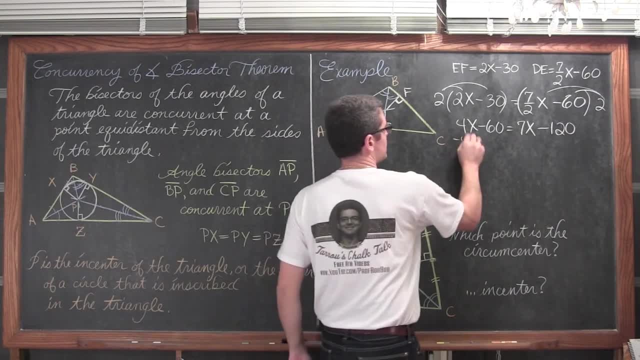 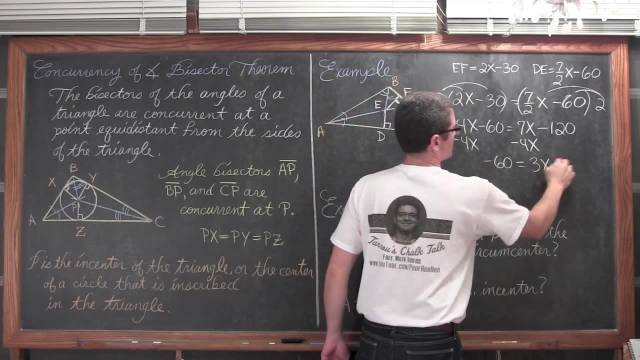 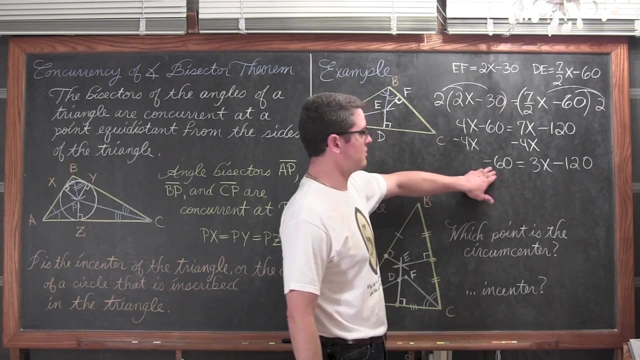 the left over to the right. So I am going to subtract both sides by 4x, We get negative. 60 is equal to 3x minus 120.. I am trying to solve for x. I am trying to get it completely isolated. So we are going to bring this 120 over to the other side. I am starting to run. 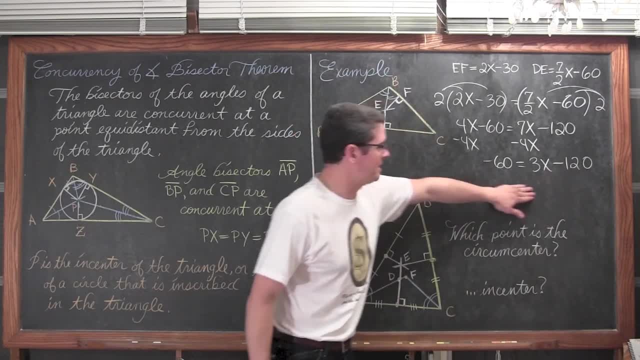 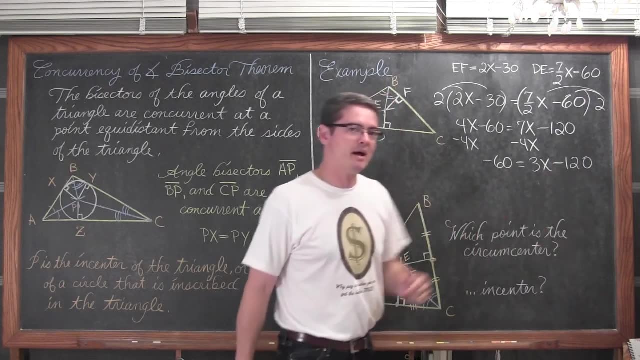 out of room. So I am just going to verbally say that I am going to add both sides by 120 to move the subtraction of 120 away from the x, Doing the opposite math operation. So negative 60 plus 120 is going to be equal to 60.. 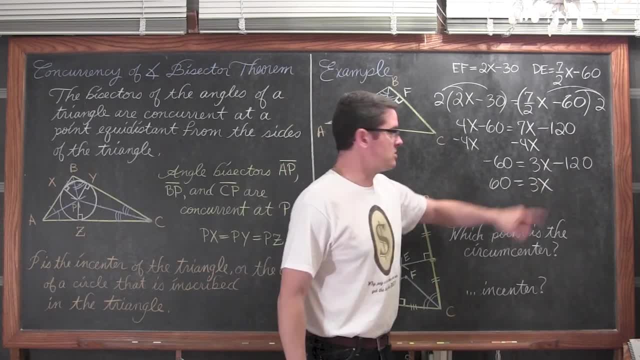 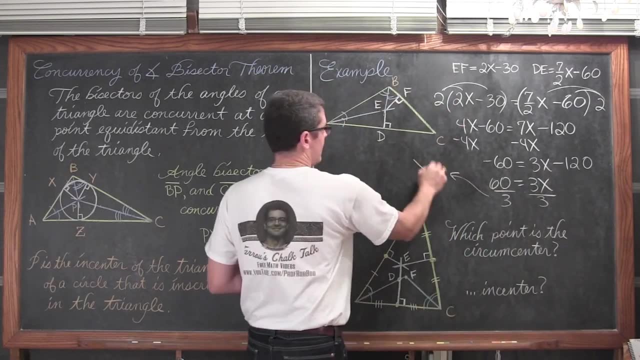 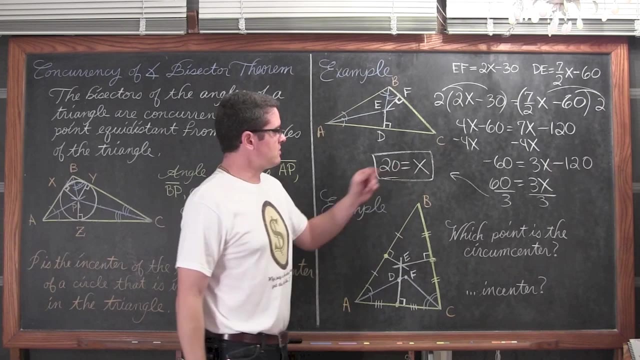 I am going to undo that multiplication of 3.. I am going to undo that multiplication again by doing the opposite math operation. So dividing both sides by 3. We get that x is equal to 20.. It is always a good idea to check your work If I want to make sure that. 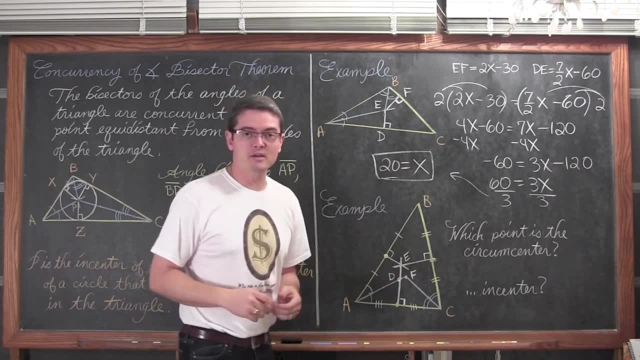 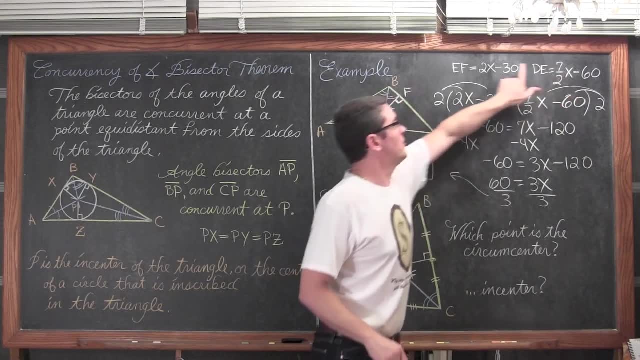 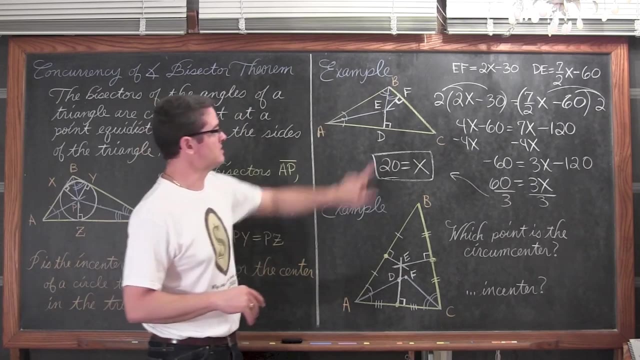 20 is right. besides glancing down at my work that I have pre-done to make this video, I am going to take this value of 20 and plug it into the original equation, or plug it into both of my original expressions. Make sure that they are equal, because they are both radiuses of the in-center. These: 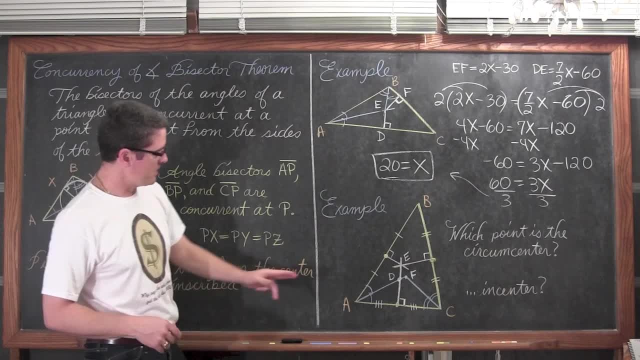 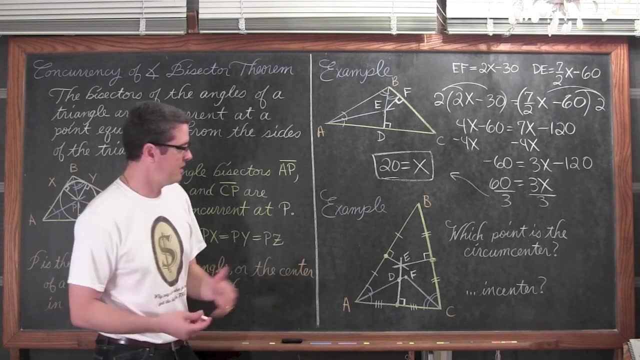 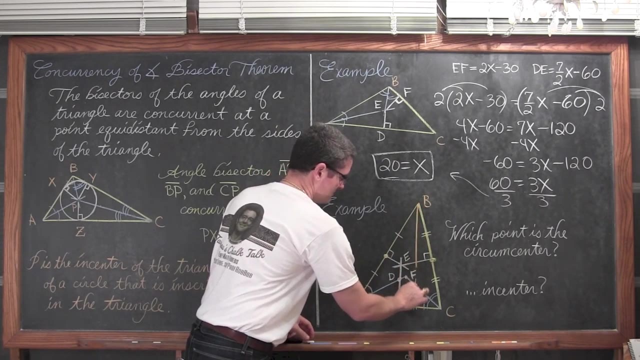 two distances are equal. Our last example: here we have triangle ABC. Let's see I wasn't trying to be too tricky by bringing in an extra line. I guess I could add it now. Let's just randomly add in that line B. what are we going to use? BG? 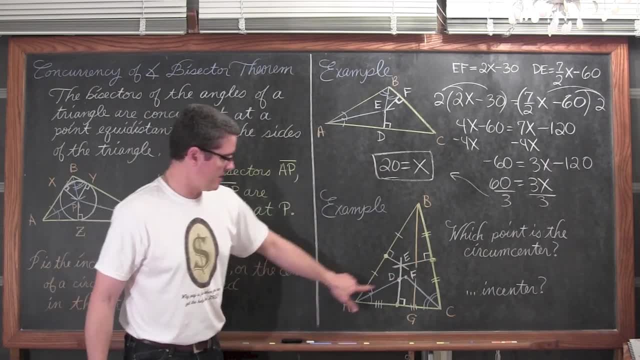 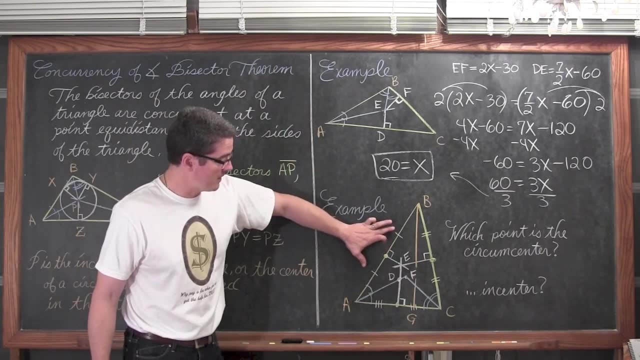 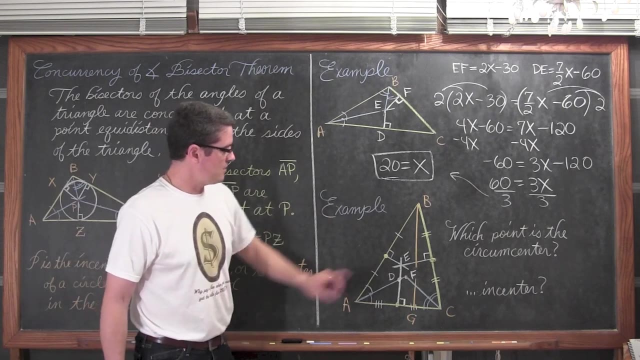 Ok, so we have an angle bisector of AD or AF, We have an angle bisector of CF, We have a perpendicular- and this would be no special point if these were not equal- but we have a perpendicular bisector, So we have a perpendicular bisector of. I guess I should have labeled.